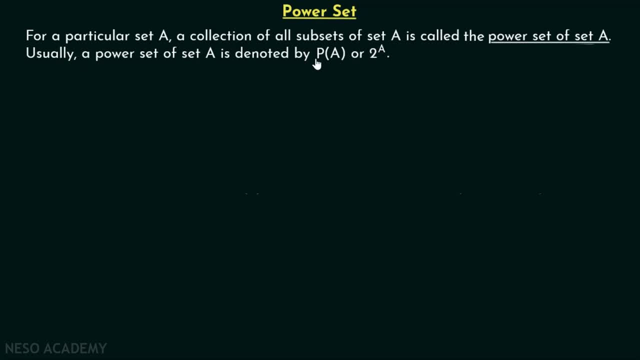 Usually a power set of set A is denoted by P A or 2 to the power A, Or we can say that P A is equal to all x, the set of all x, such that x must be the subset of A. 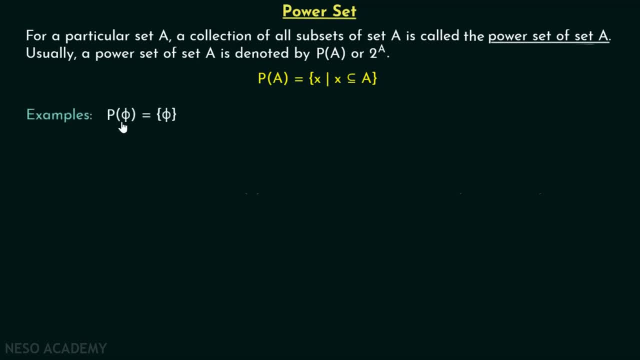 Okay, Here are some examples. First of all, if we want to find out what is the power set of phi, then this must be phi itself, Right? This is very simple, because we know that there is no element inside phi, Right? 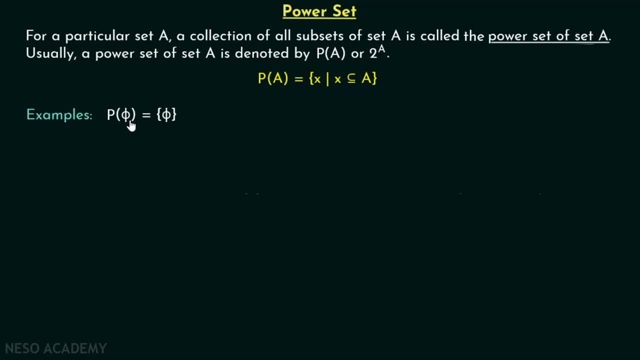 Phi is actually an empty set and we know that there is no element inside empty set, Right, And we also know that phi is a subset of any possible set. Actually, phi is a subset of every set. Therefore, phi must be there inside this power set. 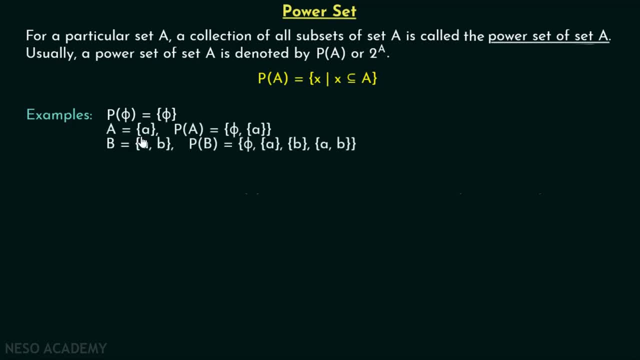 Isn't that so? If we say that A represents this set, that is this set which consists of just one element, then the power set of A must be phi and the set itself. We know that phi is a subset of every set. 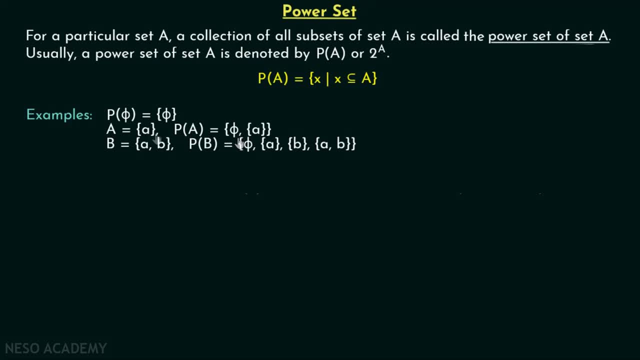 So it must be included. Apart from this, we also know that this set is itself a subset of this set. Right, This holds true because we have seen this from the theorem which we have seen in the previous lecture. Right, So phi is a subset of this set, obviously, and this set is itself a subset of this set. 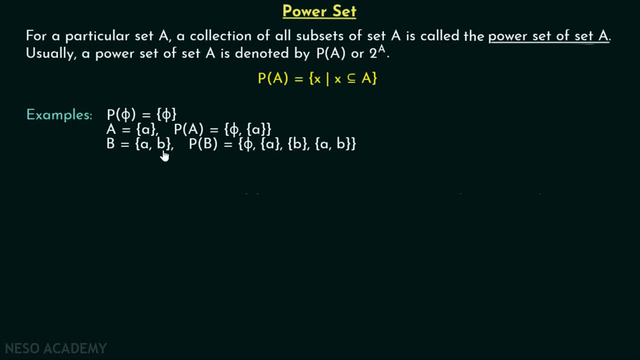 Right Now let's see this particular set B, which consists of these two elements, A and B. Now, what are the possible combinations you can make from this set? Obviously, phi must be a subset of this set and this set itself must be a subset of this set. 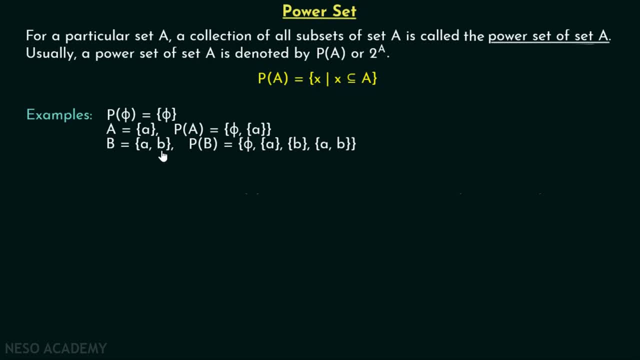 Apart from this, you can form the sets with just one element Right. Here you can see I have formed the sets with one element Right. These are subsets of this set. Obviously they must be included in this set. So we have total four elements in this power set. that is, phi A, B, A, B. 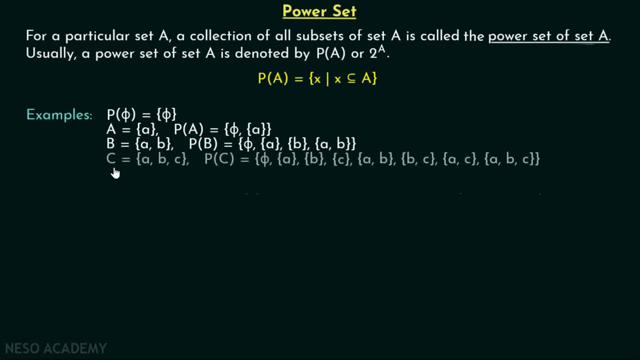 These are all the combinations possible, Right? Also, we have a set C which consists of three elements: A, B and C. Now, what is the power set of this set? Obviously, phi must be a subset of this set. Apart from this, this set itself must be a subset of this set. 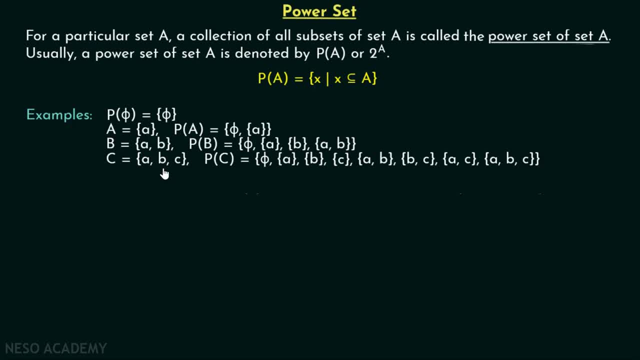 Also, we can form subsets with just one element and two elements. Here you can see there are three possibilities with one element in the set Right You can see that these are the three sets: A, B, C. Apart from this, we can form sets with two elements. 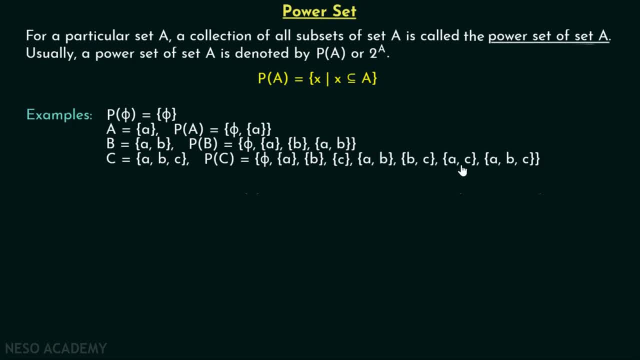 And these are the possible combinations: A, B, B, C and A C Right, And obviously the set itself must be included. So here you can see there are total eight elements in this set Right Now. you can see one pattern here in the number of elements. 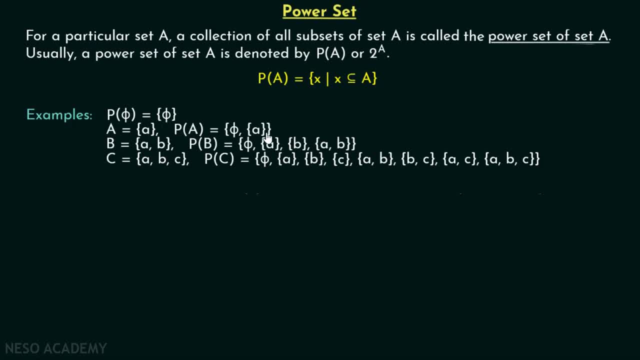 Here in this power set, we have just one element. Here we have two elements. Here we have four elements. Here we have eight elements: One, two, four, eight. You can see the pattern right. It seems like it is two to the power, something. 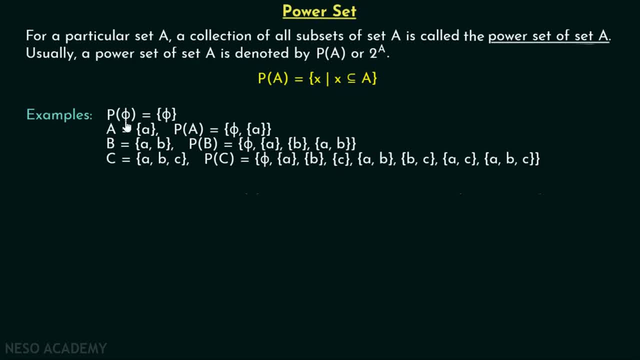 Right Here. you can see, in the empty set we have no elements. that is zero element. So here in this set we have two to the power: zero elements. that is one. Here in this set we have just one element. 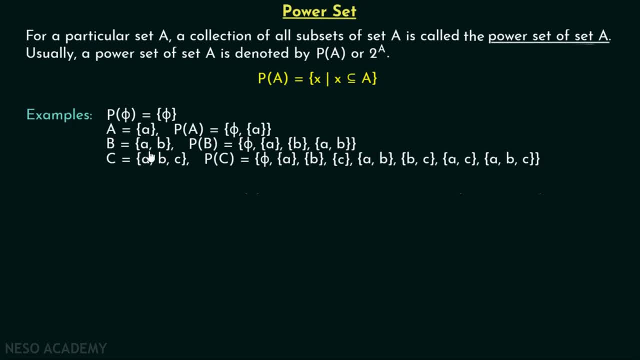 And here we have two to the power one, that is two elements. Here in this set we have two elements, And here we have two to the power two, that is four elements. Here in this set we have three elements, And that is why here we have two to the power three, that is eight elements. 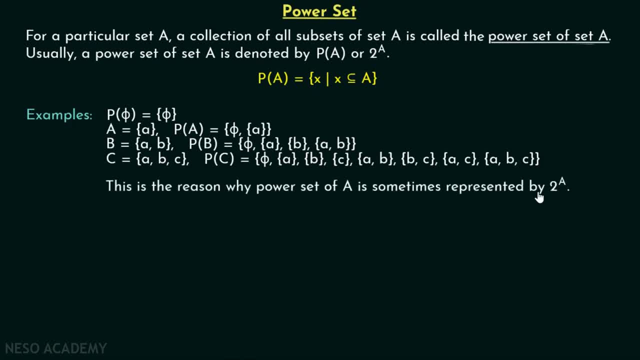 This is the reason why power set of A is sometimes represented by two to the power A. Here you can see that power set of A is also represented by two to the power A right In set A. we have only one element. In this set we have one element. 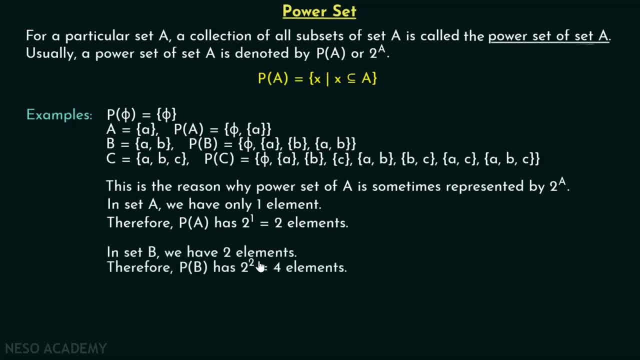 Therefore P A has two to the power one, that is two elements. In set B we have two elements, you can see. Therefore P B has two to the power two, that is four elements. Therefore, if we have n elements in set A, then P A, that is power set of A. 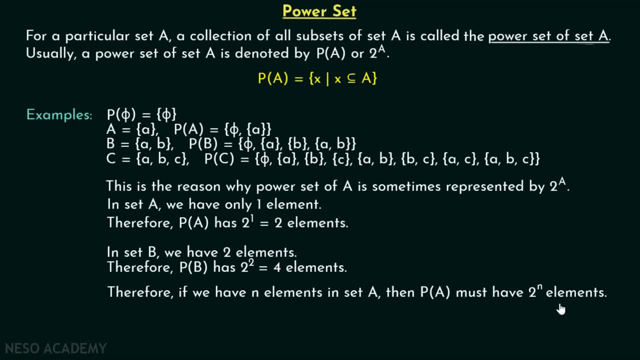 must have two to the power n elements. This is clear, right? So if I have a set with ten elements, then you know that power set of that set must have two to the power ten elements, right? This is clear, isn't that so? 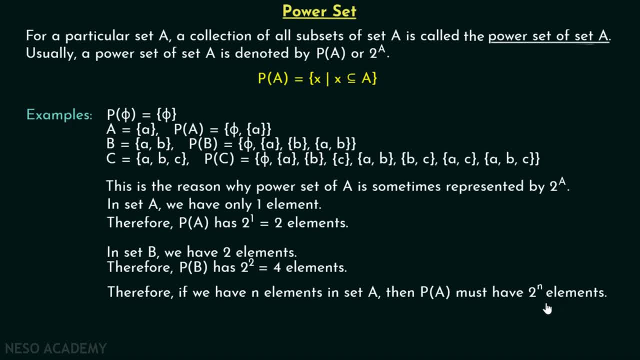 And this is what we should always remember about power set: Always remember that power set of a particular set is always a collection of all subsets of that set. okay, And also we should remember this fact that if we have n elements in a set, A. 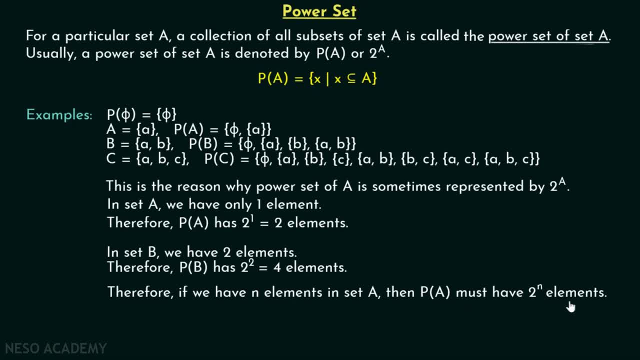 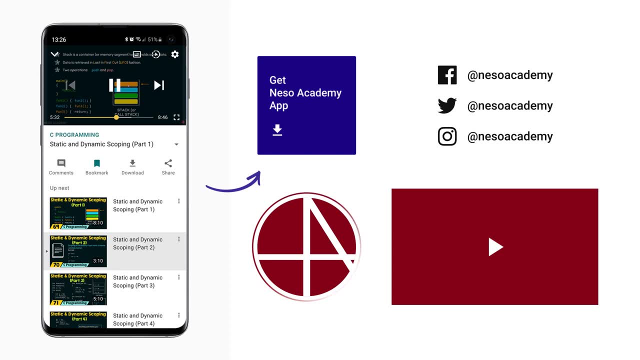 then P A must have two to the power n elements. So if we have n elements in a set A, then P A must have two to the power n elements.